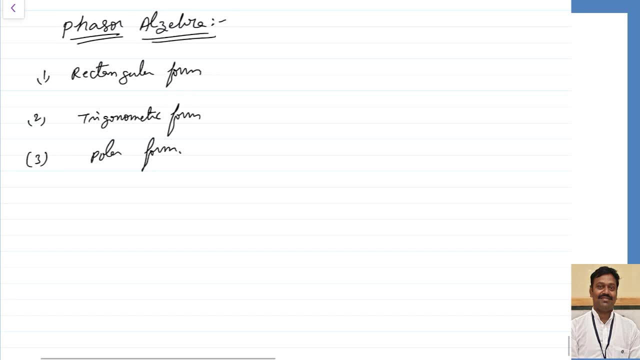 will see what are the applications for the phasors. So once these basics are clear, so next class we will discuss about the application to the AC circuits. So first let us assume I have this because x-axis, y-axis coordinate system can be represented like this: Let us assume one phasor. 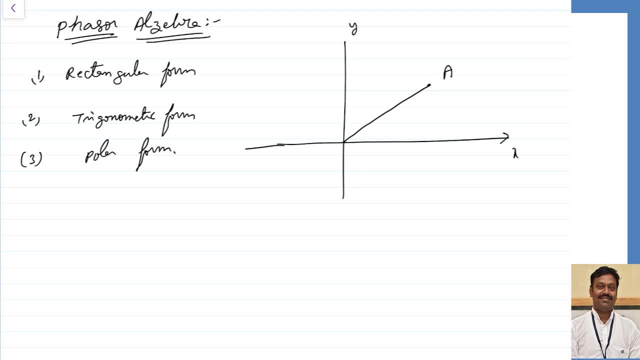 is there, whose magnitude is 1.. Let us assume having a magnitude of a1, because this is the rms value, So it is represented like this. Let us assume it is displaced with respect to x-axis in counterclockwise direction, So phi1. 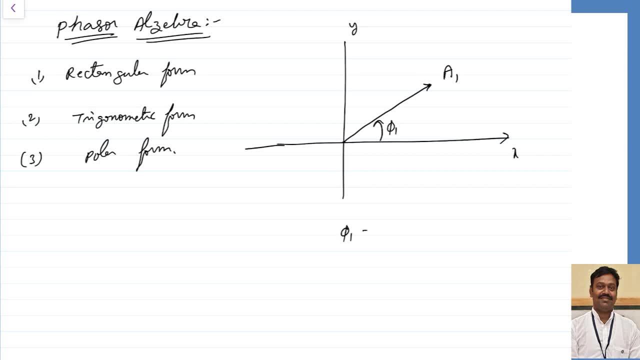 is the angle bit. angle phi again is the advancement of phasor from x-axis in counterclockwise direction. We have to take in counterclockwise direction. Let us assume a phasor a is there which is having an angle of phi1 or which is leading the x-axis. 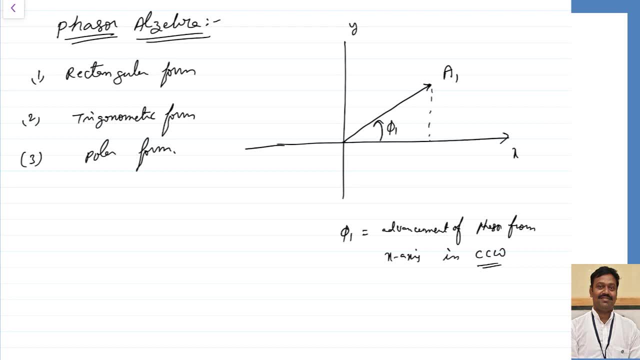 by angle phi1.. So this can be resolved into two components, one along the x-axis and another one along the y-axis. Let us assume the component in the x-axis I am representing with a. this will be nothing but a1 into cos phi1. 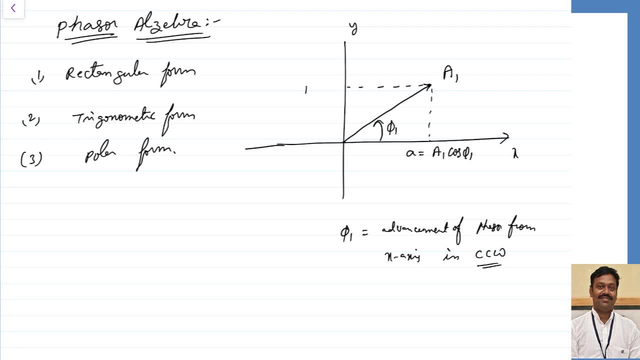 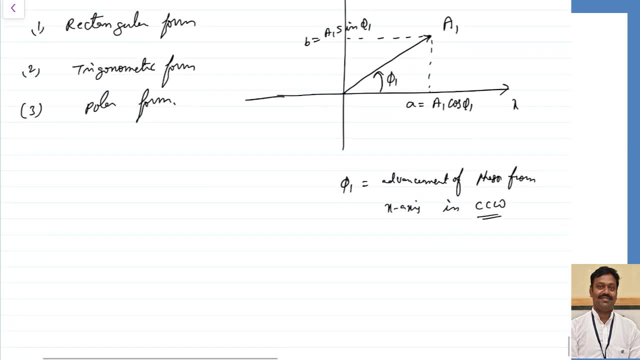 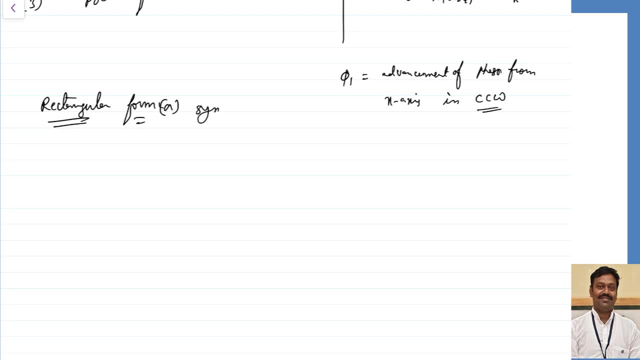 because from this we can calculate. so similarly, the y-axis I can calculate. the value b is equal to a1 into sin phi. So let us use these basics to represent each of these things. So first I am starting with rectangular form. So in rectangular form this is also called as the symbolic form, because it can be represented. 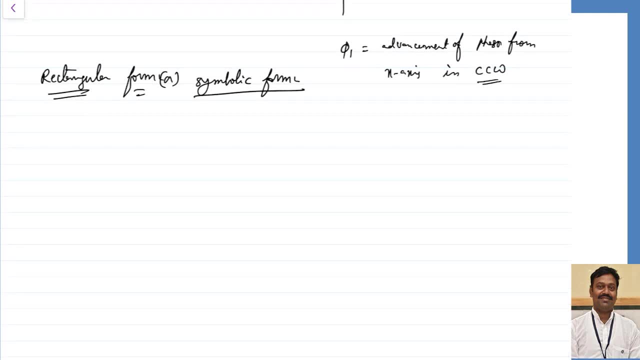 in the symbolic form, So in the rectangular symbolic form, the vector, whatever vector you take, it will be represented in the form of the x component, plus or minus j times of the y component. Let us take, for example, if I am taking this, phase r, so this can be represented as the 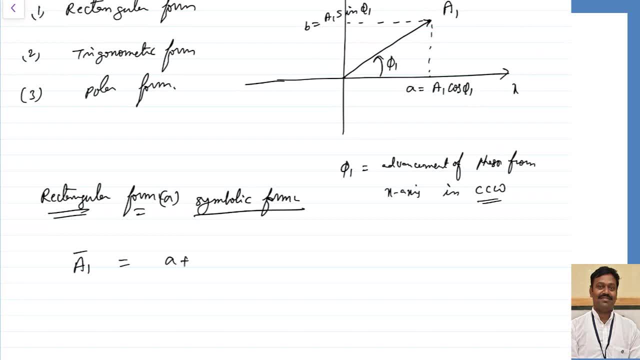 phase r will be equal to a plus jb. a plus jb. This j indicates imaginary axis or the y axis. So if it is in the positive y axis, then this will be plus sign. If it is in the negative y axis, then this sign will become minus, or this I can represent. 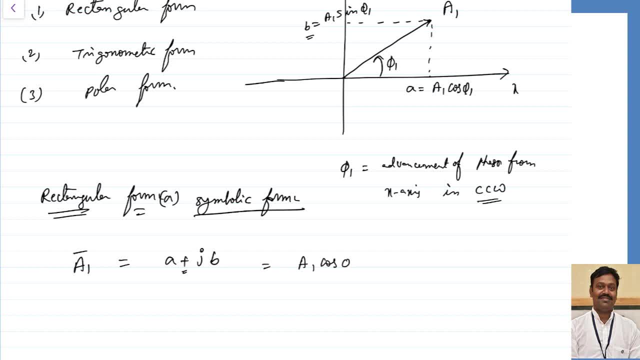 as This is nothing but a1 cos phi1 plus j times of a1 sin phi1.. So just substitute the values, then you will get this value. So if you want to get the magnitude, so magnitude, let us assume any value is specified in rectangular. 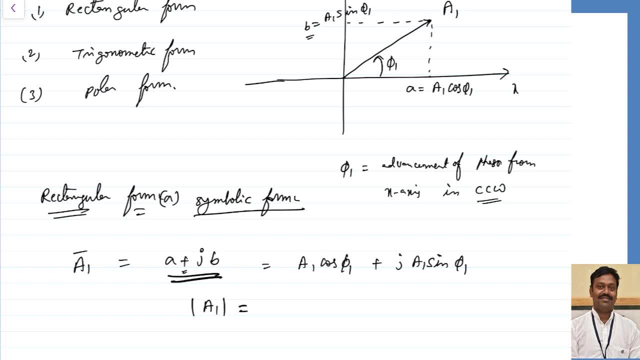 coordinate system and I want to calculate its magnitude. the magnitude will be equal to square root of a square plus b square, And the angle or the advancement with respect to the x axis will be equal to tan inverse of b by a. So using this, we can calculate. 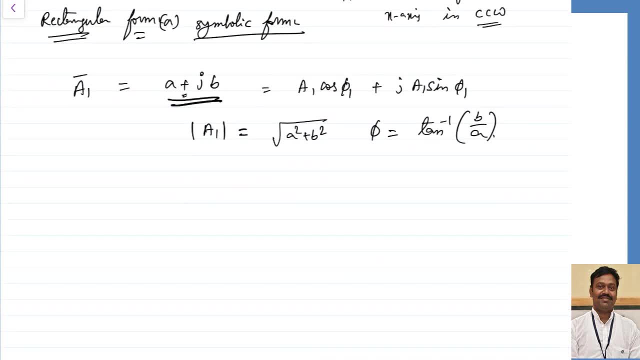 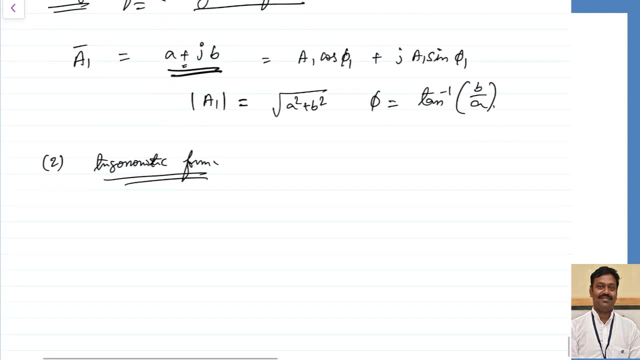 As this you have already studied, so I am not going into deep. My concern is only application part. So the second form, which is called as the trigonometric form- all these forms look like one- is something similar to the second one because they are correlated. only these are. 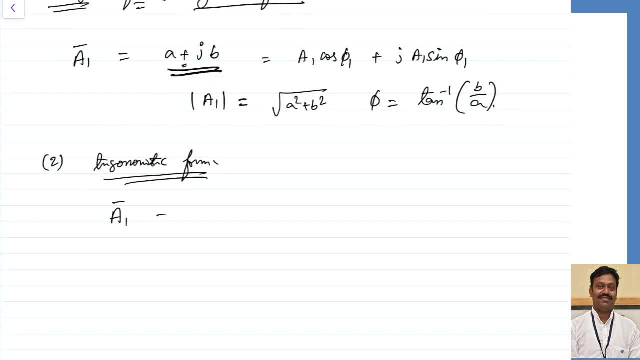 different ways of representation. In trigonometric form, this vector will be represented in the form the a1, the magnitude multiplied by cos phi1. That means this will be represented as the phase r in terms of cosine wave and the sine wave plus j sin of phi1. 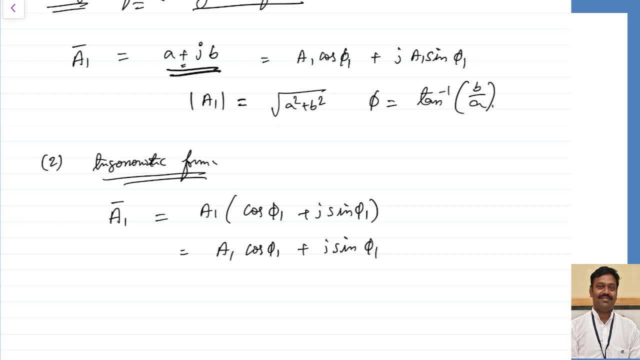 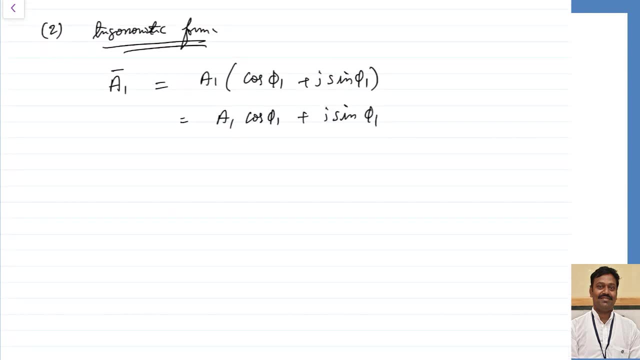 So what does this mean? Because both rectangular and these are related to be together. So we will take the example. So in the examples it will be clarified, just to try and understand how they are representing. So details we will see in numerical. 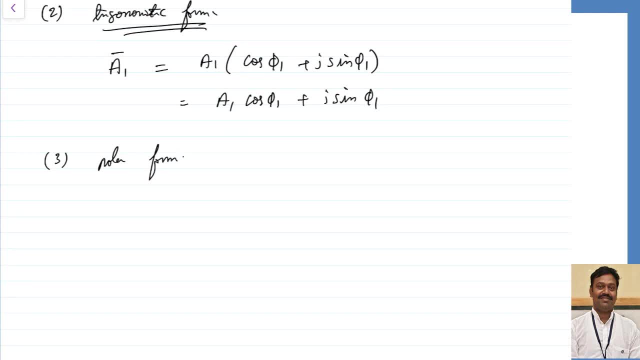 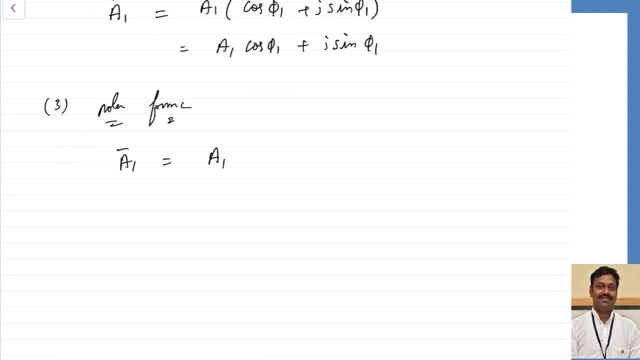 So third form is called as the polar form. So in the polar form, So in the polar form, The phasor is represented by the magnitude of the phasor. phasor I am just representing with the normal letter. it indicates the magnitude, followed by the angle of the phasor. 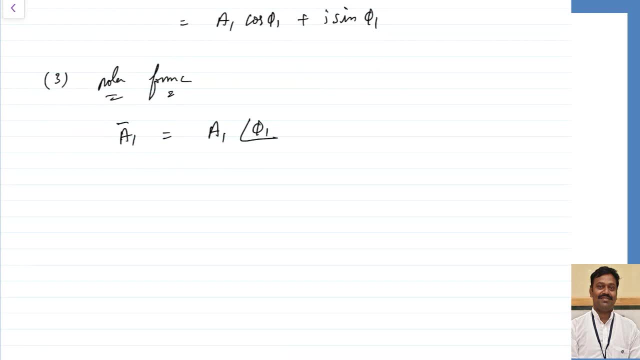 So how much it is advanced with respect to the x axis. So how to get this? if rectangular coordinate system is given? if you want to calculate in polar coordinate system, the magnitude will be equal to square root of a square plus b square. So, as per the previous one, then phi I can calculate by tan inverse of b by a. 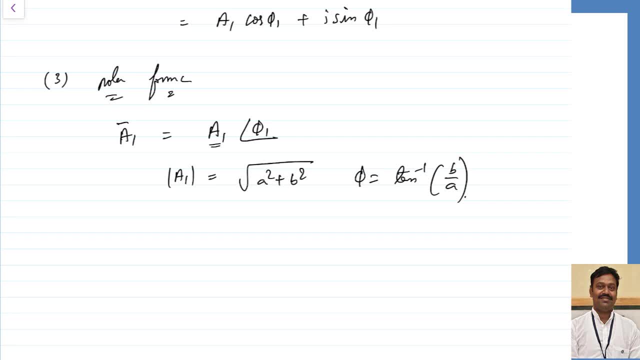 So let us assume I want to convert from rectangular coordinate to polar coordinate, polar coordinate: what I have to do? I have to do square root of a square plus b square and phi. I can calculate by tan inverse of b by a. Now I want to convert from polar to rectangular coordinate system. 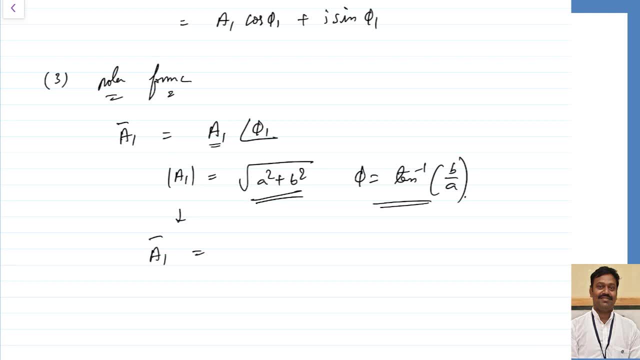 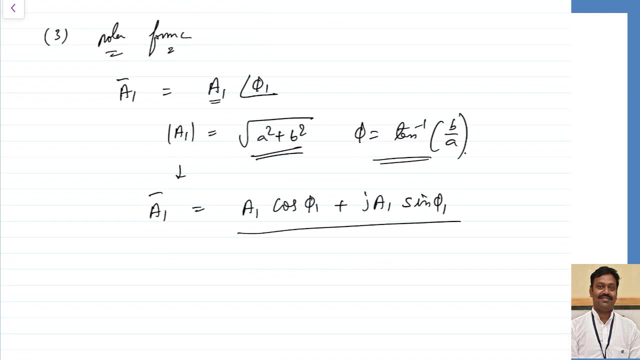 If I want to convert this to rectangular coordinate system, this I can obtain as just write the magnitude into cos of the angle plus j sin of j a1 into sin of the angle. So this gives my rectangular coordinate system, Or It is something related to trigonometric. 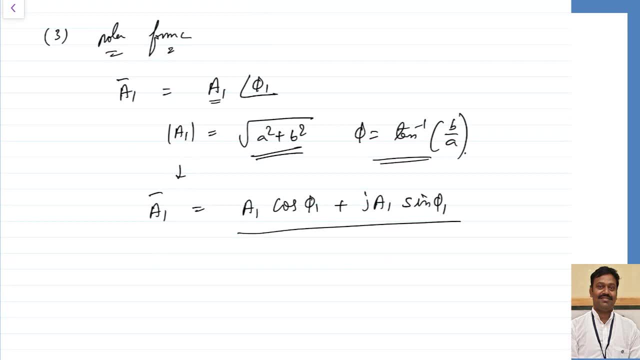 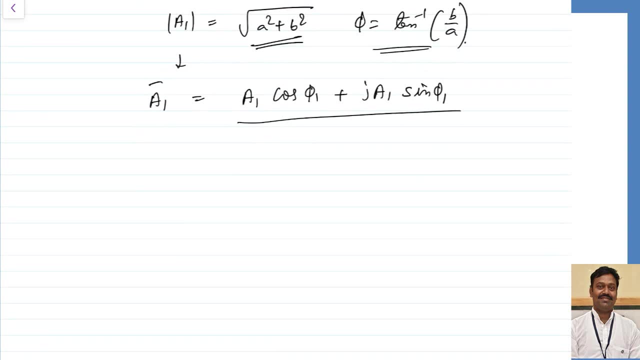 That means, if you are not substituting the values, it is called as trigonometric. If you are substituting the values and simplifying it, it is called as the rectangular coordinate system. Let us try to take one example so that these coordinate systems will be clear to you. so 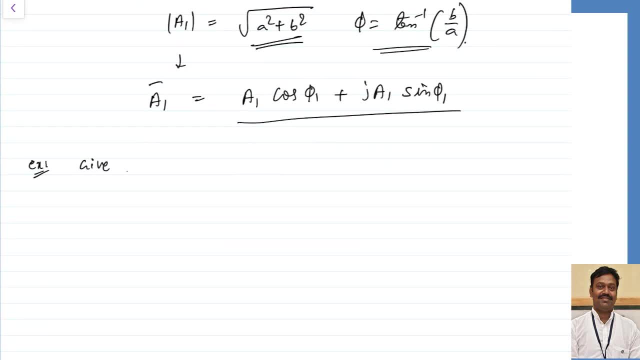 that I can proceed further. So it is asked: give the voltage expressed in the symbolic form. Symbolic form: V is equal to 5 plus j12 volts in trigonometric and polar forms. trigonometric and polar forms. So how to solve this? 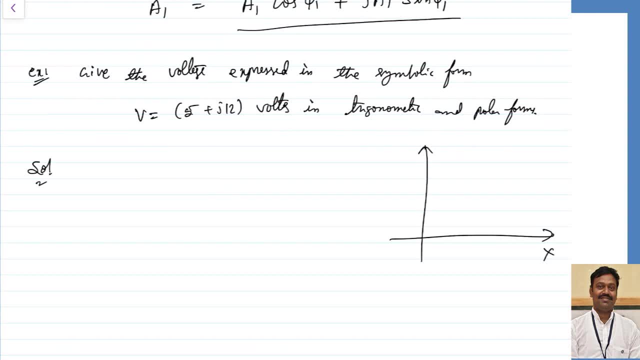 So this can be solved like this. So let us try to represent this in the coordinate form. Coordinate form: It is written there 5 plus j12. That means in the x direction it is having 5 units and in the y direction it is having 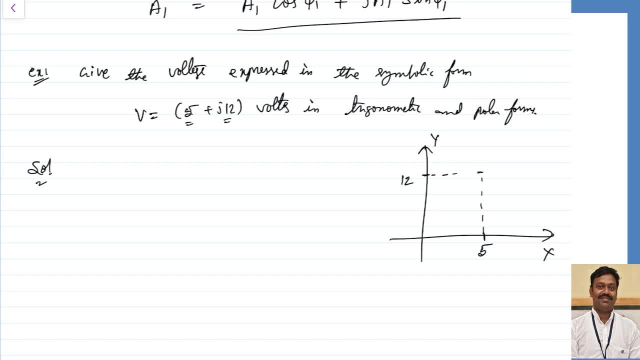 12 units. So you just extend these two, They will intersect at a point. That intersection gives you a tip of your phasor. So this is the tip of my phasor, which is represented by V. So the advancement with respect to x axis I can represent by angle phi. 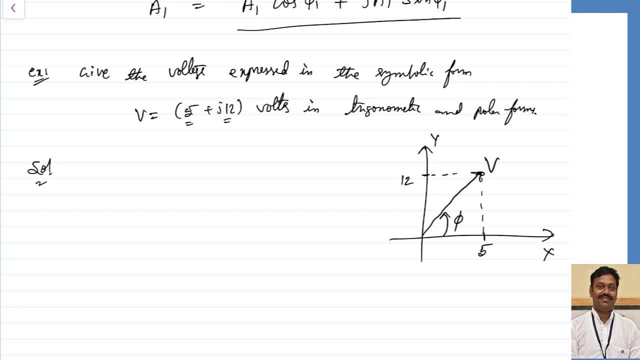 So let us see how to convert in the other forms. So from this I can calculate the magnitude of my phasor will be equal to square root of x square plus y square, x component square plus y component square. So this will be equal to 13 volts and the angle I can obtain by tan inverse of y component. 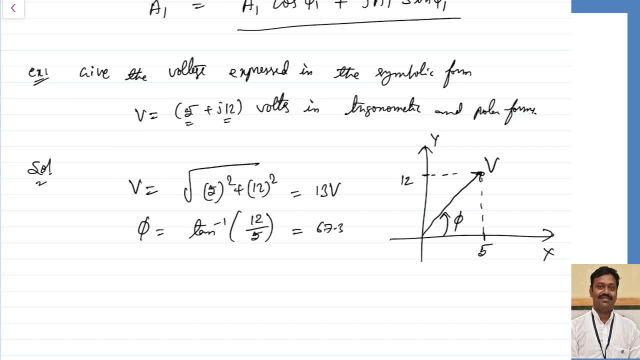 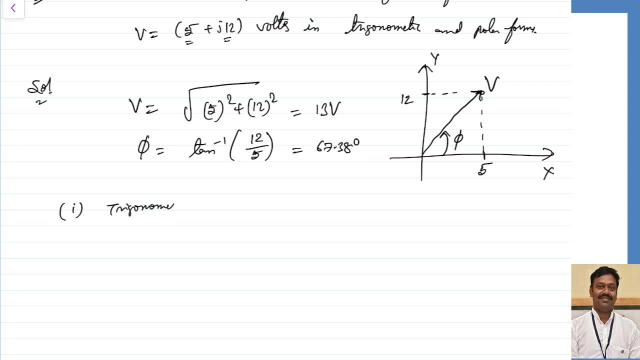 by x component 12 by 5.. So this will be equal to 67.38 degrees. This is what we obtained. So let us now represent in trigonometric form. So trigonometric form this will be equal to vector. V is equal to magnitude into cos. 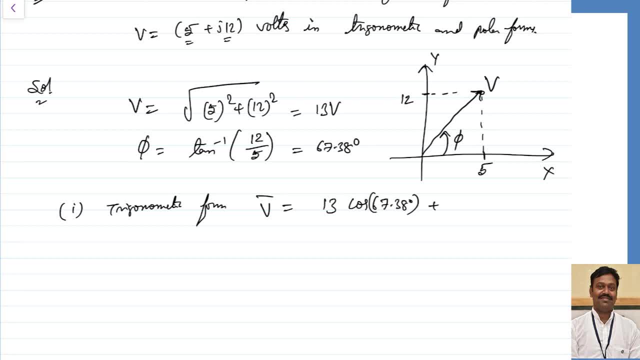 67.35.. 37.38 degrees plus j 13 into sin 67.38 degrees. You are not substituting the value you are representing in the cosine wave and sine wave form, So that is why it is represented like: 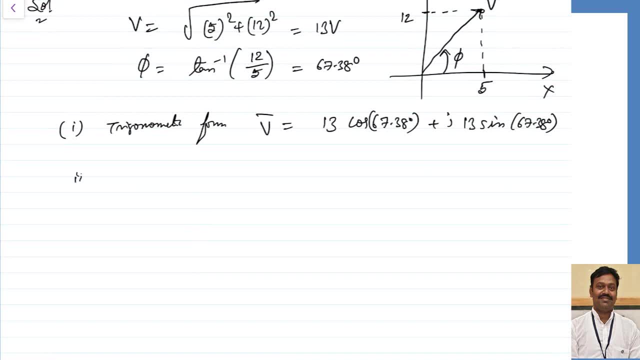 this. This is called as trigonometric form. So then the second one. it is asked: calculate in polar form. So if you want to represent in polar form, polar form will be nothing but the magnitude, and we have to write the angle. The angle is 67.38 degrees, So in 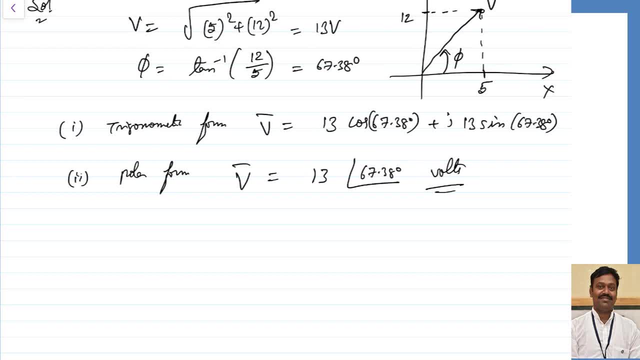 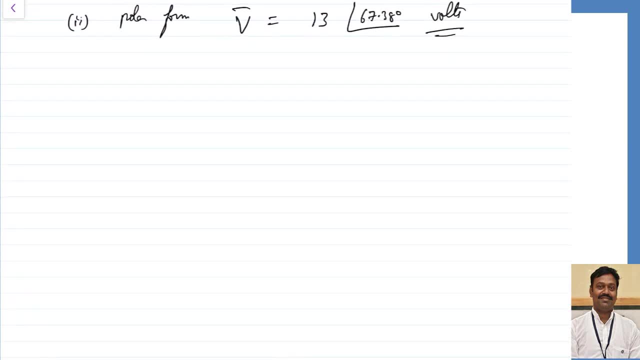 this way we have to represent. So I hope that trigonometric form, polar form and the rectangular form are clear to you. So let us now see how to do the addition and subtraction of a phasor, and which method will be better out of all. So now, addition and subtraction. 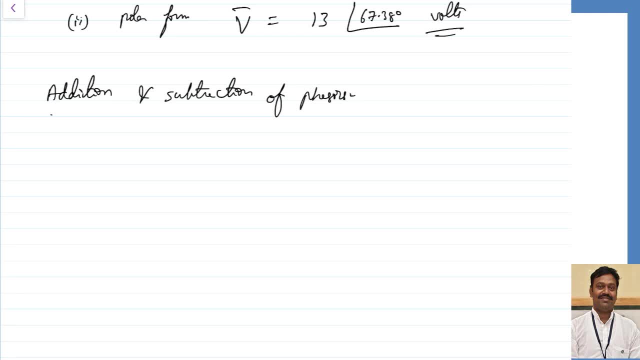 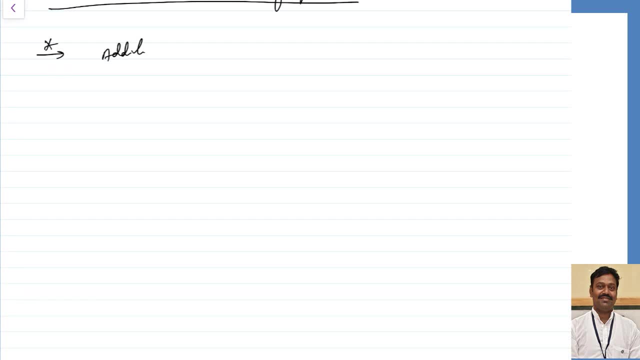 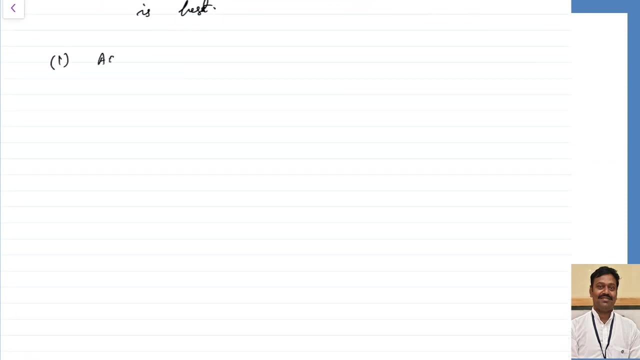 of phasors. So one thing you have to remember here: the thumb rule for addition or subtraction, Rectangular form is best out of all. Rectangular, or it is also called as symbolic form, best. The reason is it is very easy to calculate. Let us see it First. I am starting with addition. 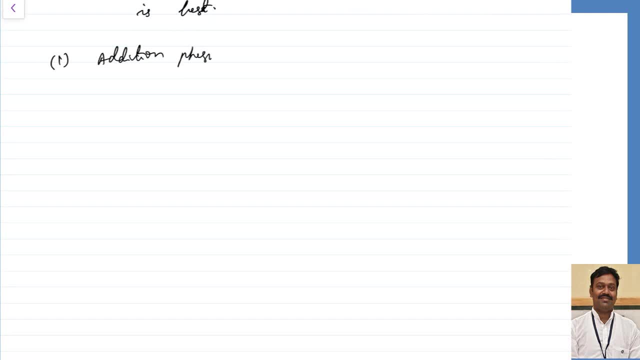 of phasors. So I am just taking the coordinate system. I am taking two voltages. Let us assume there are two voltages. One voltage is v1,, which is having an angle of theta 1,, which is leading the x axis by theta 1 degrees. I am taking another vector. this vector is v2,, which is 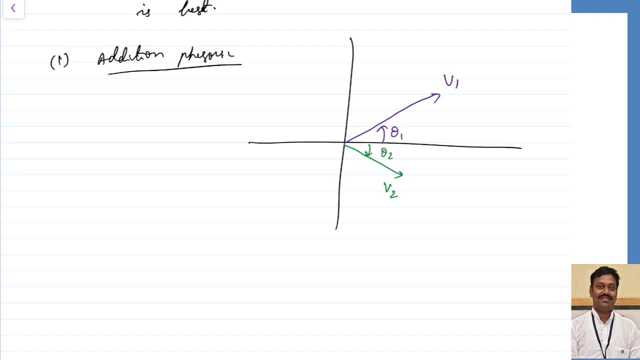 lagging behind the x axis by some angle, theta 2. Lagging means no hangings So we can, just means we have to take the angle as minus. remember this. so each of these vectors can be resolved into x component and y component. so i am just trying to resolve each of this component, this v1. i am. 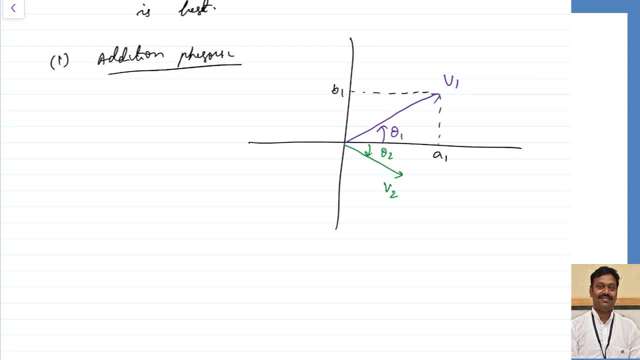 resolving into x component. this becomes a1, this becomes b1. similarly, this v2, i can resolve into two components. one is along the x direction. x direction is a2 and y direction is b2. you remember here, because in this direction it is plus, this direction it will be minus. so this becomes minus. 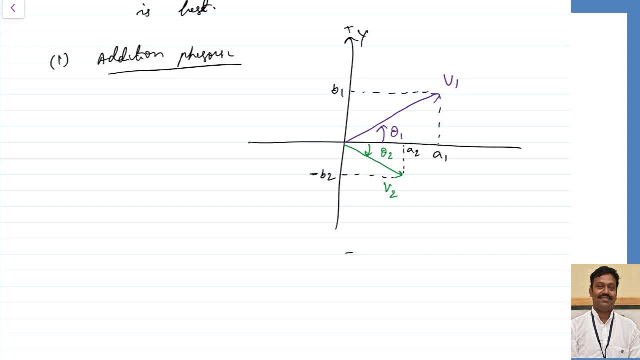 b2. remember this. so i have resolved this into two components, so let us try to solve it. so here, v1 i can represent as a1 plus jb1 because, resolving into this, similarly, v2 i can represent as a2 plus jb2, or this can be represented in follower form as these are vectors in the phasors. so v1. 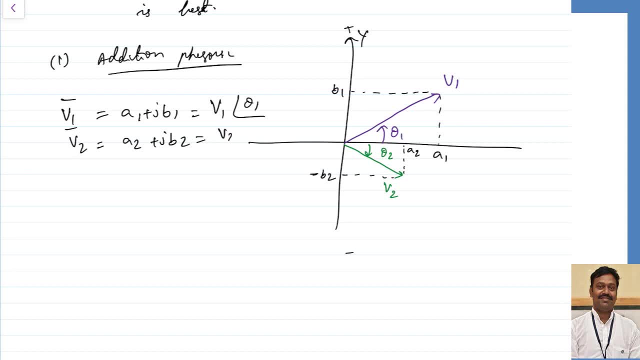 at an angle of theta1 and v2 will be v2. at an angle of minus theta2 because it is lagging behind the x axis, or we are moving in clockwise direction. if you are moving in clockwise direction, you have to take it as minus. or if you want to convert from rectangular to polar or polar to, 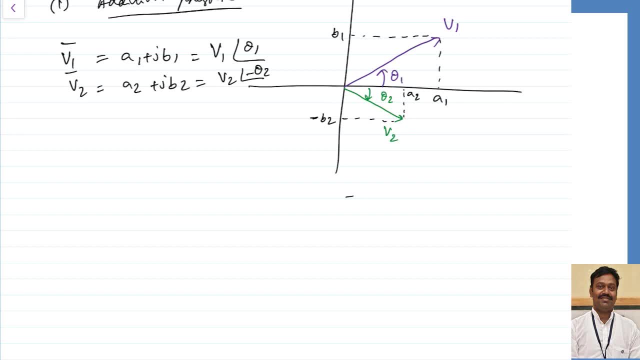 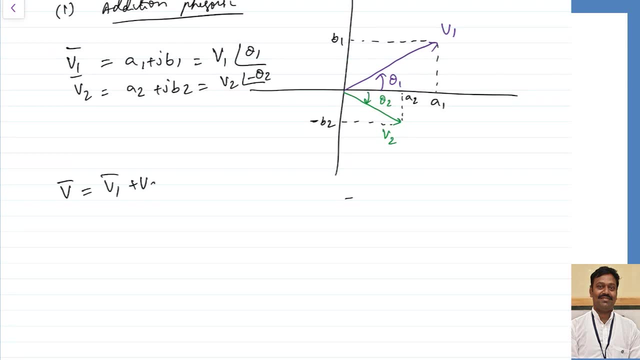 rectangular coordinate system that can be converted easily. we have already seen it. so let us see what will be the sum of the vectors. so if you want to take the sum of the voltages, that is v1 plus v2, let us see in rectangular coordinate system because it is easiest. if you want to add this, 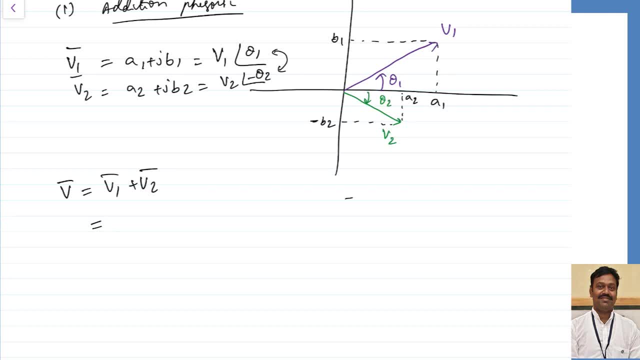 polar coordinates, magnitude plus angle. it is very difficult task. you have to convert to trigonometric form, then add them and then again bring them. that is a lengthy process. so that's why let us try to solve directly with rectangular coordinate system: a1 plus jb1 plus a2 plus it is a2. sorry, here it is. 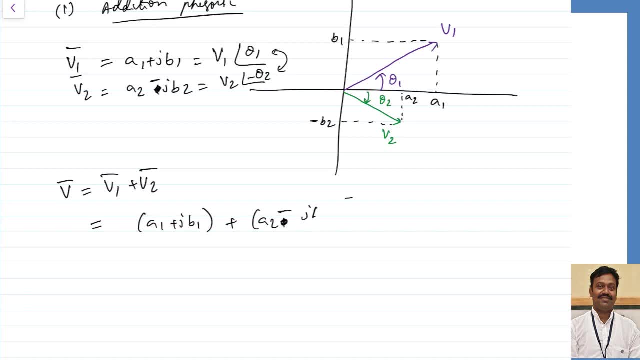 minus right, minus jb2, minus jb2, because it is in minus y axis. remember this. so this will become a1 plus a2 plus j times of b1 minus b2. what i have done? i have just added the x component. i have just added this. 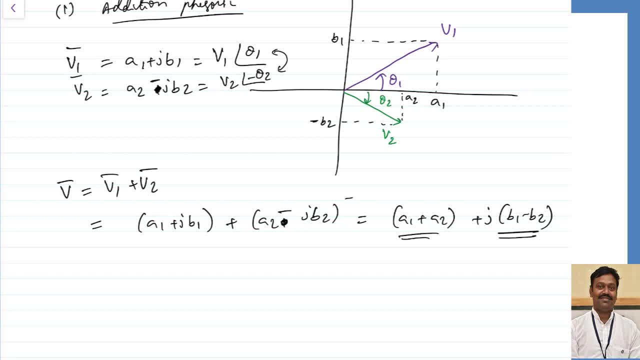 because i have just added the x component. i have just added the x component. i have just added this, the y-components. This give my resultant. It is that much easy. So once the resultant is done, we can just convert it to polar form or any other form we want Similar way. let us see the. 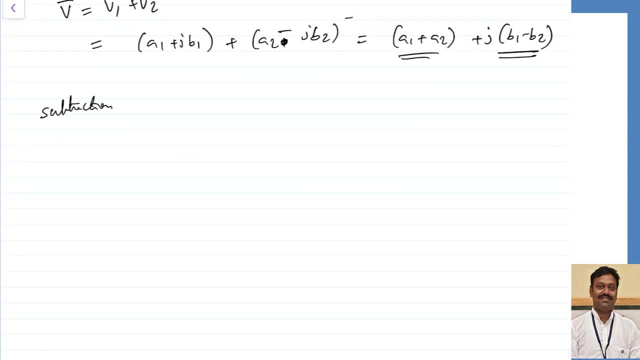 subtraction of phasors. Subtraction of phasors. So let us assume I want to calculate: v is equal to v1 minus v2.. So same way I can calculate a1 plus jb1 minus a2 minus jb2 in this example. 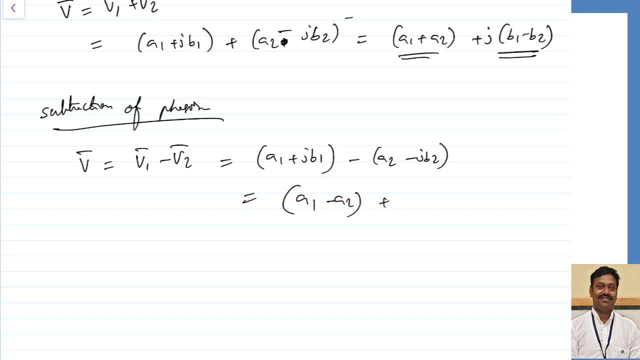 So this will become a1 minus a2 plus j times of b1 minus of minus b2.. So this become b1 plus b2.. So this way we can calculate very easily. Now coming to the multiplication and division of: 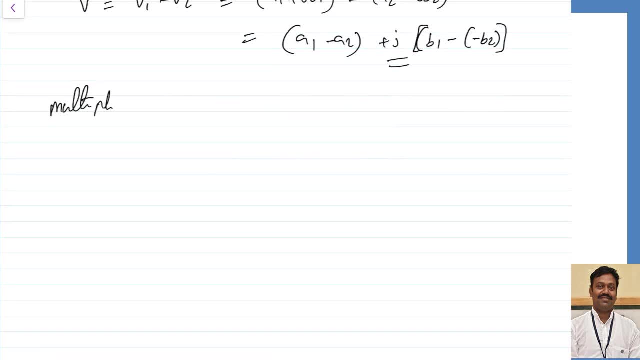 phasors. So if you want to do the multiplication or division. So we are going to prove that the polar form is best for this. Polar form is best for this. Let us try to derive it so that then we will make the summary. So first let us start with. 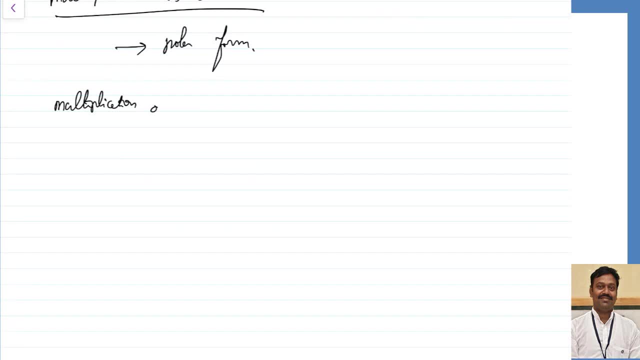 multiplication of phasors. So for multiplication of phasors, let us again take the same, whatever the phasor we have taken, that is, a1 plus jb1 and the value of v2, let us take it as a2 minus jb2 minus j is there, or this is nothing but the value with the angle, and this v2 is nothing. 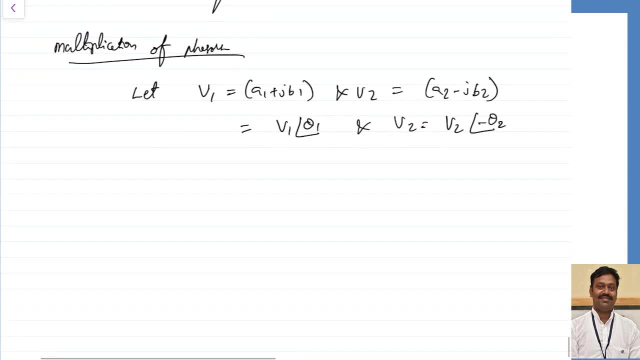 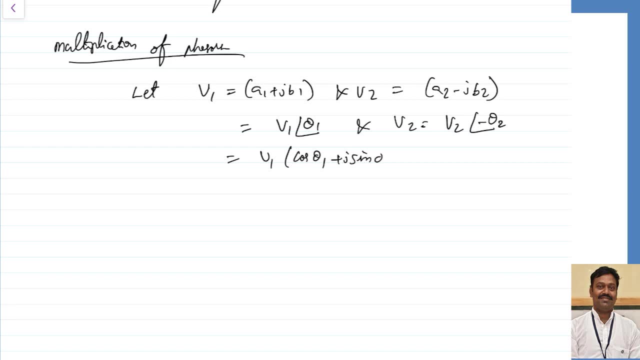 but v2 at an angle of minus theta2.. Getting it or this trigonometric form I can represent as v1 cos theta1 plus j sin theta1, and this v2 I can write as v2 into cos theta 2 minus j sin theta2.. 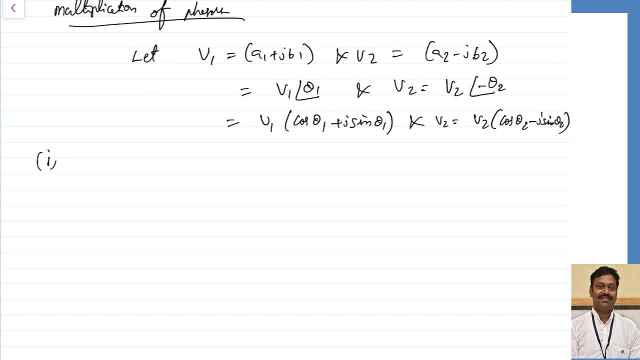 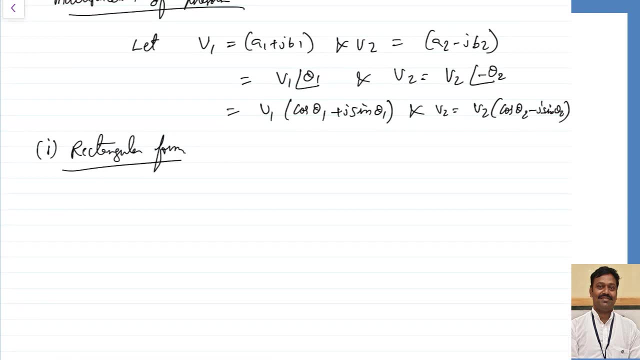 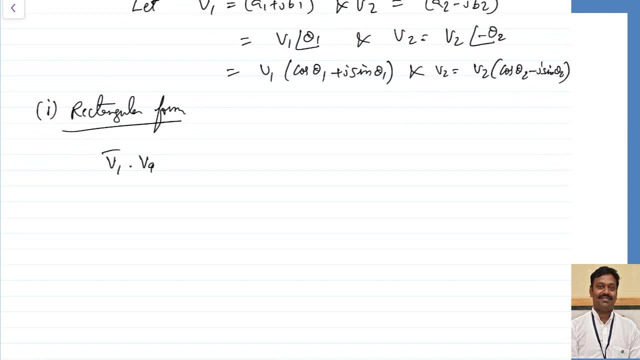 This I can represent. So now let us solve it using rectangular form. So remember, the rectangular form is obtained from the trigonometric form only, and the vice versa, because all are correlated to each other. So I want to multiply v1 multiplied by v2.. This is my target. So v1 is a1 plus j, b1.. I have to multiply with a2 minus j. 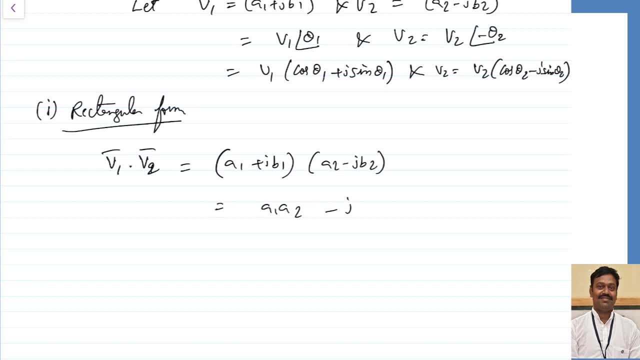 v2.. So this will become a1- a2 minus j1 times of a1, b2 plus j times of a2, b1 minus j square times of b1- b2.. So this I can write as a1- a2.. This j square because, remember, here j is nothing but. 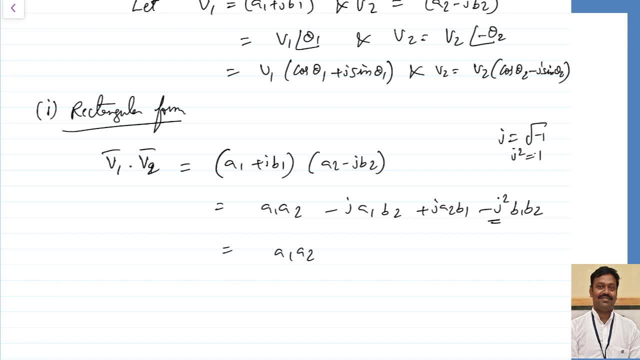 square root of minus 1, or I can write: j square is equal to minus 1.. So this one I am just substituting here: j square is equal to minus 1.. So minus of minus becomes plus. So this becomes b1, b2 plus j times of a2, b1 minus a1, b2.. So this way we have to solve. This is the case only when. 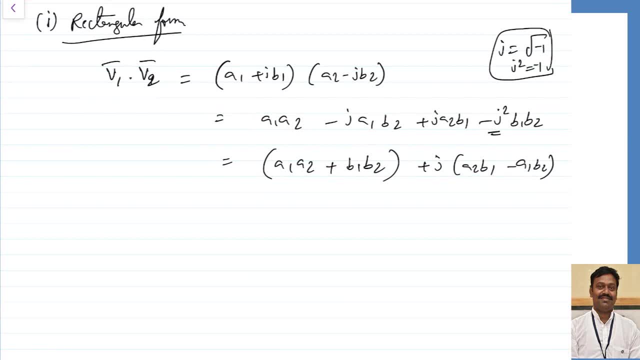 two are there. If multiple are there, it becomes much more complex. So let us try to solve using trigonometric form, So trigonometric form. it will be much more complex. So trigonometric form, So trigonometric form. if I want to multiply v1, 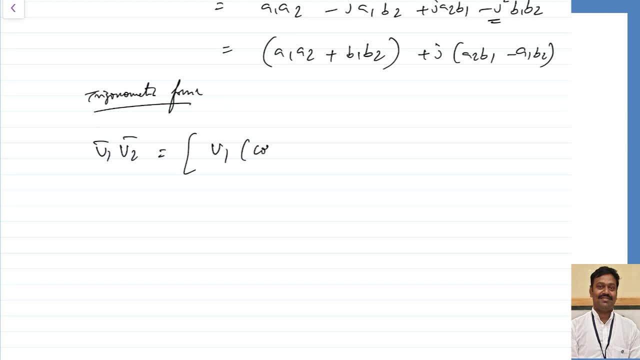 multiplied by v2, this will become v1 into cos theta 1 plus j, sine theta 1.. This I have to multiply with v2 into cos theta 2 minus j sine theta 2.. This minus sign is because angle is negative, So this becomes v1: v2 into cos theta 1, cos theta 2 plus sine theta 1, sine theta 2 plus. 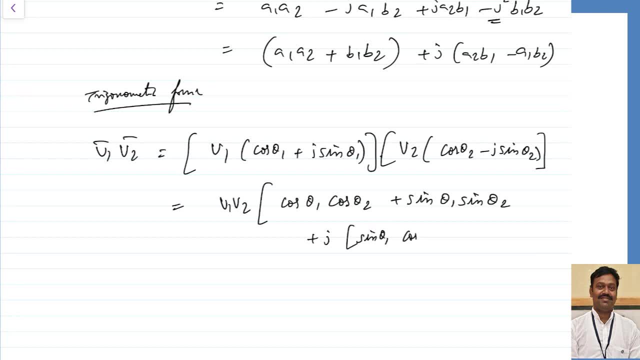 j times of sine theta 1, cos theta 2 minus sine theta 2 into cos theta 1.. This is what we get if we simplify it. Or this I can write as: v1: v2 into cos a, cos b plus sine a, sine b. This will: 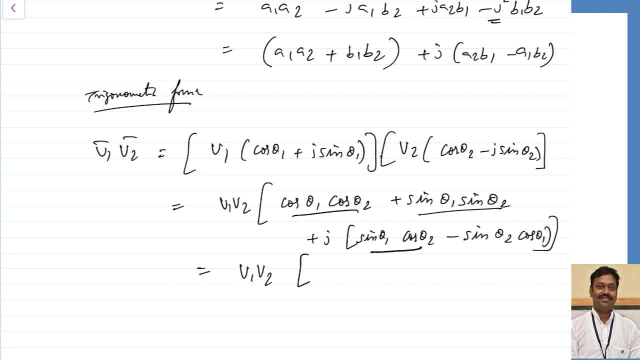 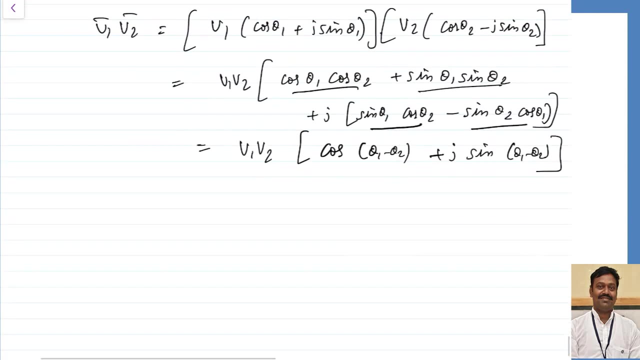 become a minus b. Similarly, this will be sin a cos b minus cos a sine b. This will become sin a minus b. So this becomes cos theta 1 minus theta 2 plus j times of sin theta 1 minus theta 2.. So this way we have to solve. Let us solve. 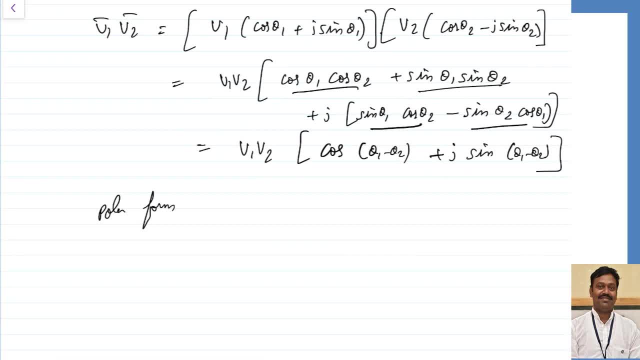 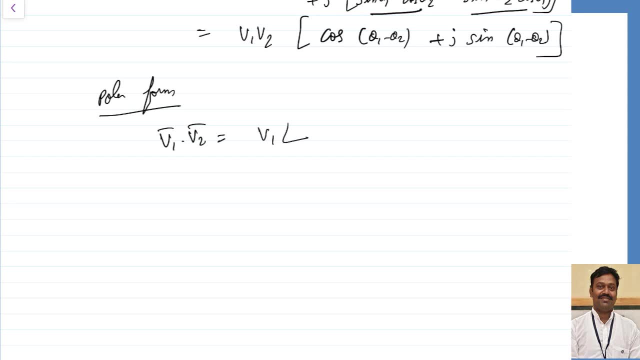 using polar form. In polar form, if you want to multiply v1 multiplied by v2, so this will be nothing: ri of theta 1 multiplied by v2 at an angle of theta 2. so how to calculate this? just simply do the. 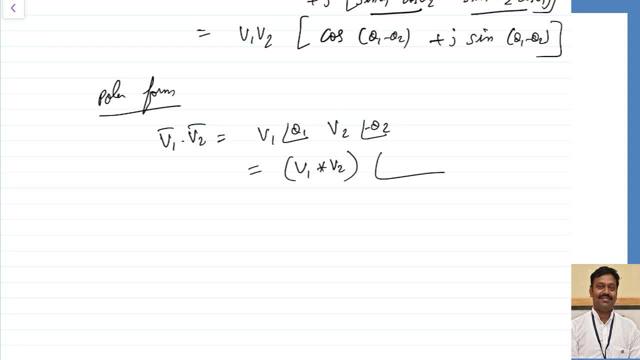 product of the magnitudes and angle, you have to directly add the angles. sorry, this is minus theta 2, right? so this is theta 1 plus whatever is the angle, theta 2. just do the addition of those things, so directly you can obtain the product using polar form. same thing is the case for the case. 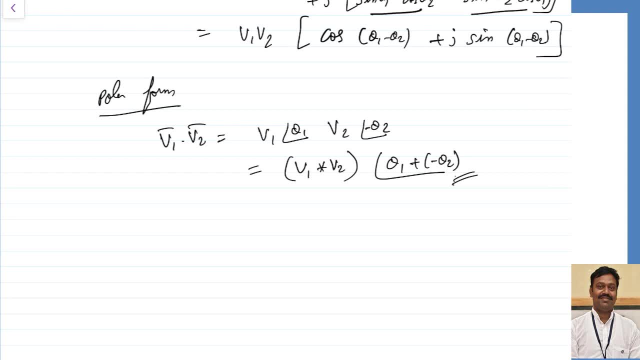 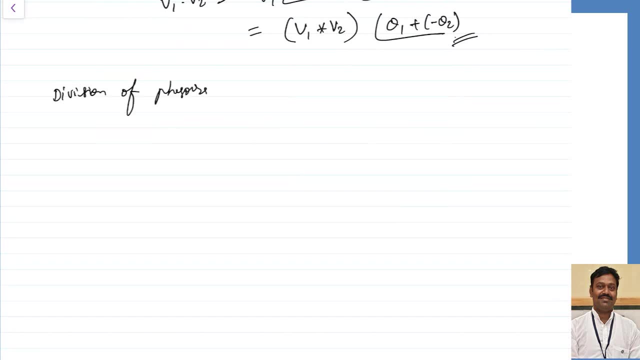 of division. for the case of division, if you want to do the rectangular coordinate system, it will be much more complex. let us see the division of phasors. in the division of phasors, if you go for rectangular coordinate system, i want to divide v1 minus v2, which will become a1 plus jb1. 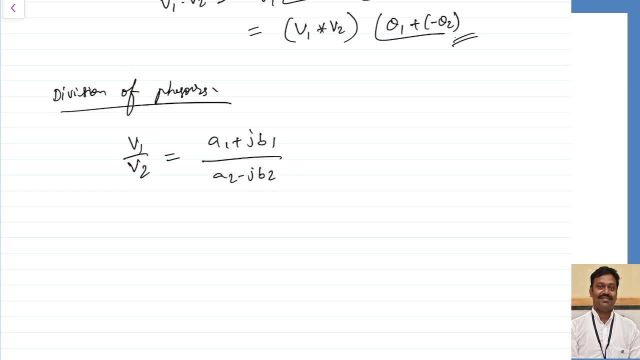 divided by a2 minus jb2. this is there. so to solve this in rectangular is very tough. so what we can do, we can multiply the numerator and denominator with conjugate of the denominator. what is the conjugate if any vector is represented by a plus jb1? 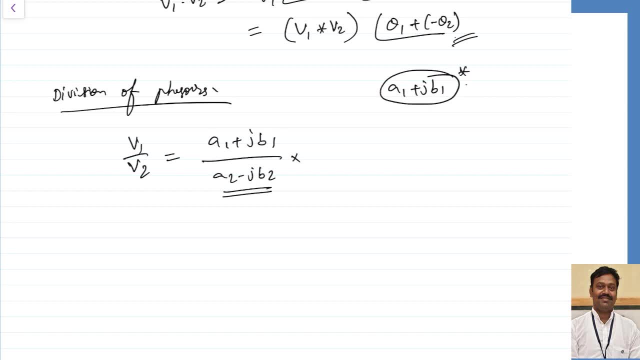 you can multiply the numerator and denominator with the conjugate of the denominator. the conjugate of this conjugate is represented by the star on the top. the conjugate will be only. there will be the sign in the imaginary component. that means the conjugate of this will be a minus jb1. 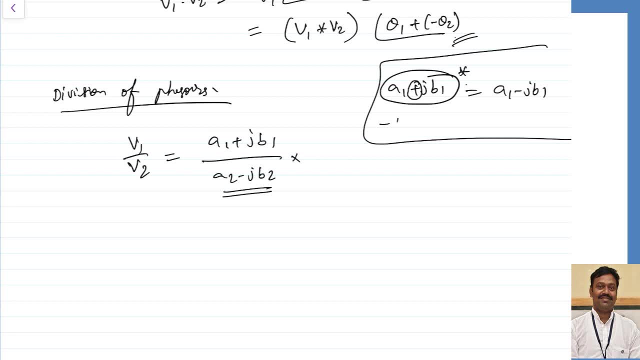 so let us take another example. let us assume i am having minus a2, plus jb2, something like this is there. i have to take the conjugate of this if i want to take the conjugate of this x component will not change, only whatever is the y or the j component, is there change the sign of that component? 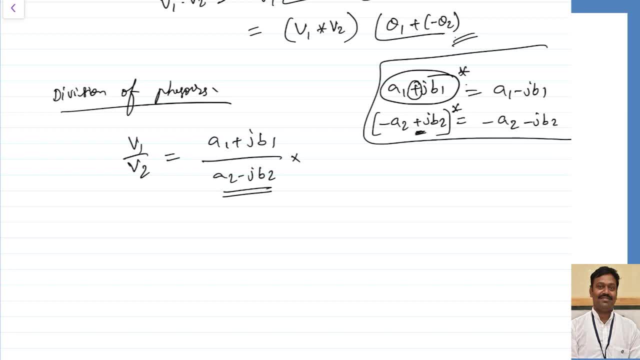 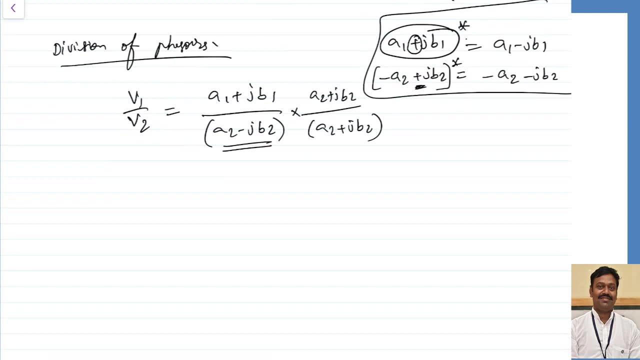 if it is minus, it becomes plus, if it is plus, it becomes minus. only that thing, you have to remember. so i am multiplying this with a2 plus jb2, divided by a2 plus jb2, so that my denominator will not have any imaginary component. all will come in the numerator. i can get my solution easily, so this you: 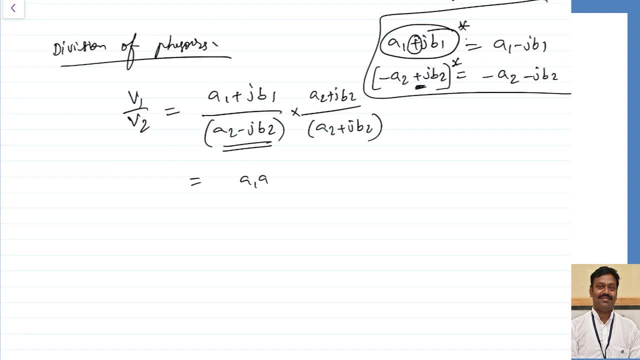 can multiply and see i am directly writing the answer. so you will get as: a1. a2 minus b1. b2 divided by a2 square plus b2 square plus jb1 b2 divided by a2 square plus b2 square plus jb1 b2. 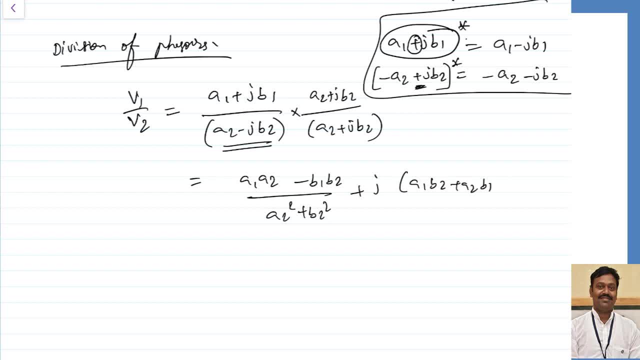 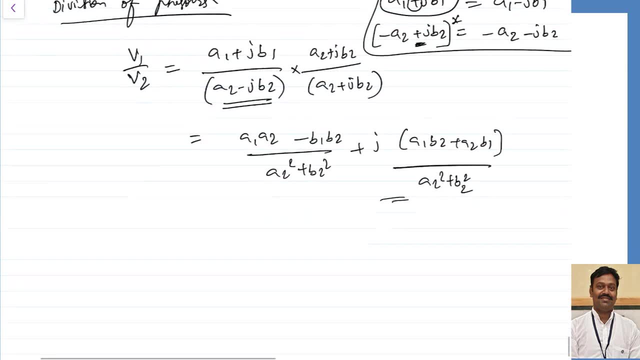 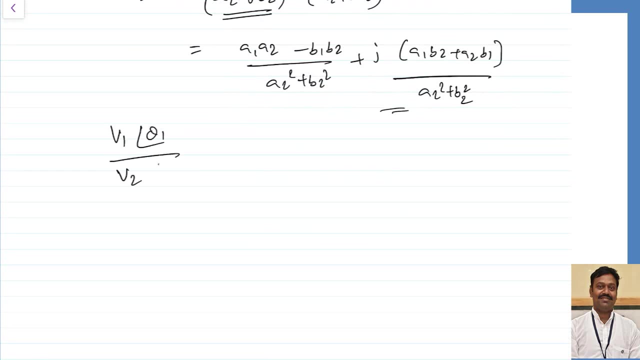 times of a1, b2 plus a2, b1 divided by a2 square plus b2 square. even if you remember the formula also, it is so much complex to calculate. but if you want to convert simple using polar form, so this will become v1 at an angle of theta 1 divided by v2 at an angle of. in our example it is minus theta. 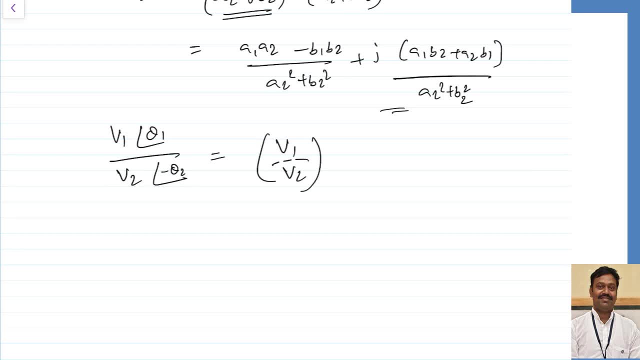 2. so you have to simply divide the magnitudes and angles. you have to subtract the theta 1 minus whatever is the value of theta 2, because in our example it is minus theta 2, so you have to. in our example it is minus, so i have written minus theta 2. it is that much easy. so let us now. 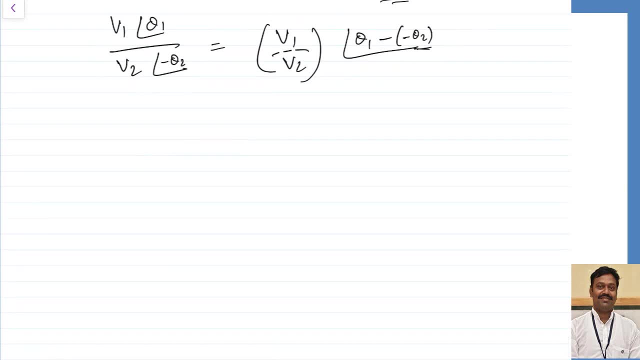 see how to calculate for the case of powers, because powers is nothing but multiple product a into a into a. in that way i am multiplying. so let us see the power and roots of phasors. so for power and root of phasors, let the value of v is given by a at an angle of theta. 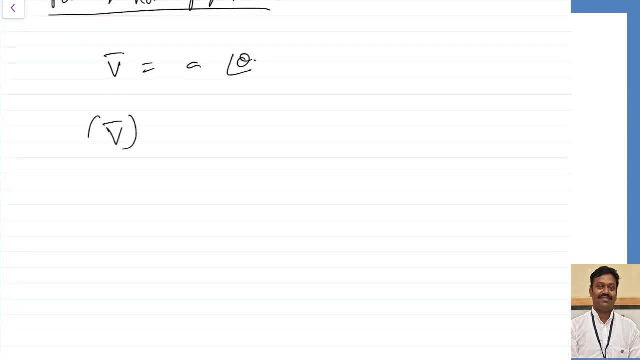 so i want to calculate for the case of powers, because powers is nothing but multiple product. i want to calculate the v to the power of x. how can i calculate? so this? i can directly calculate as a to the power of x into this theta multiplied by the power. let us take one example to clarify. 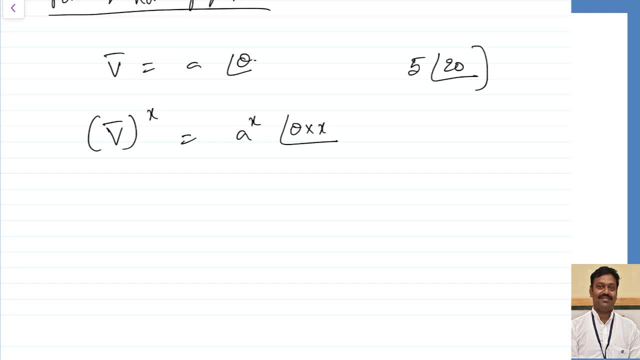 this. let us assume i have one phasor, 5. at an angle of 20 degrees i want to make to the power of 4. so how to calculate this? just take 5 to the power of 4 and in the angle you just multiply with 4. 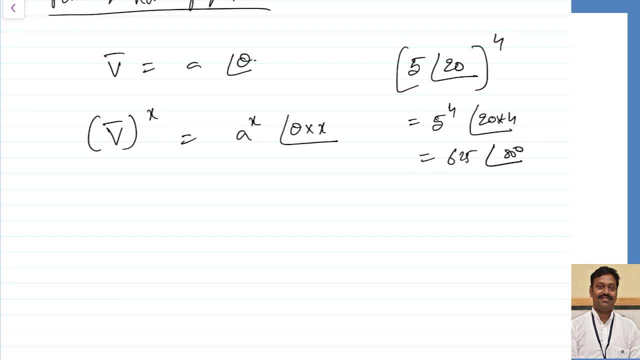 so this becomes 625 at an angle of 80 degrees. it is that much simple. so let us now see: if i want to calculate the nth root of v, nth root of v, how can i calculate this? so if i want to calculate the nth root of e, i have to. 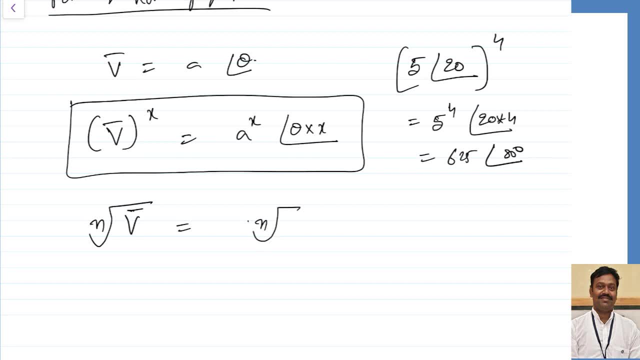 calculate the nth root of the magnitude and the angle, i have to divide with that n, that angle, i have to divide with n. let us take again an example to clarify this. let us assume i have the value 5 at an angle of 20, so i have to take the equal to n, and the angle of n is of 1.5, so i have to divide. 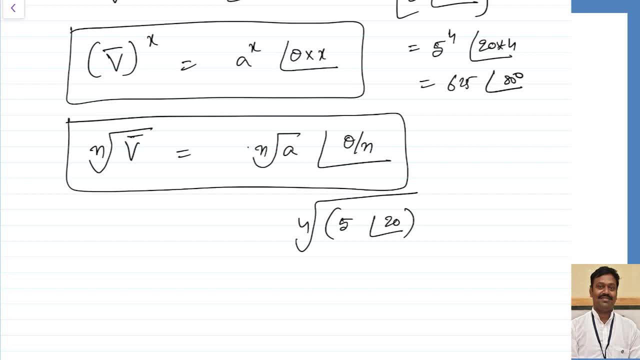 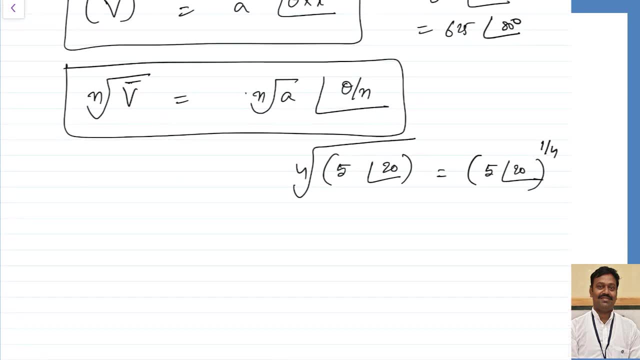 to take the fourth root of this, or to the power of 1 by 4,, because this is nothing, but this way also, I can represent- to the power of 1 by 4, because square root is 1 by 2, you already know. So this is simple: you have to just take the fourth root of 5 and 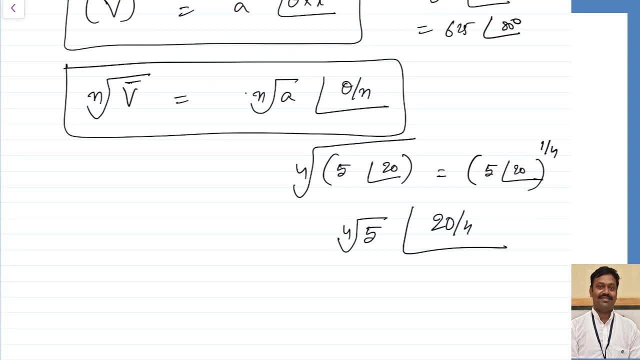 the angle. what we have to do? you have to take the angle divided by that root. that means 20 by 4.. So if you calculate this, you will get it as 1.496 at an angle of 5 by 4.. So finally, I am making the conclusion from this. then we will try to solve one or 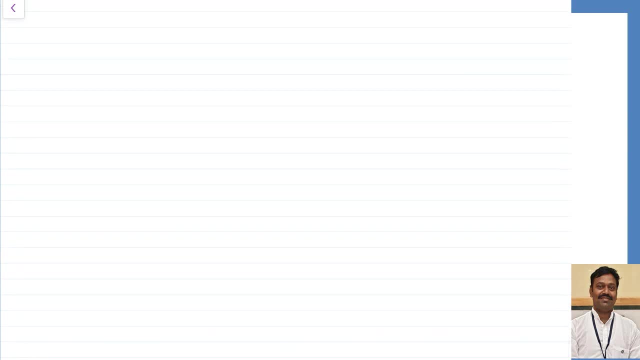 two numericals to further clarify this. So the major conclusion is: whenever you want to do the addition or subtraction, so we have to go for rectangular coordinate system, And if you want to do the division or multiplication, then you have to go for the polar coordinate. system. So in rectangular coordinate system if you want to do the multiplication then you have to go for the polar coordinate system. So in rectangular coordinate system you are going to take the square root of 4 by 4.. So you have to take the first root, that is at. 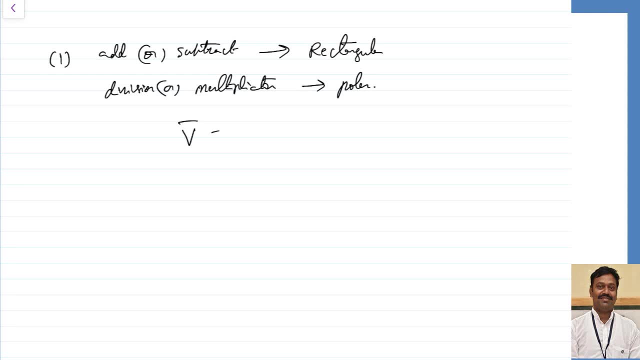 system any vector is represented of the form. the vector v is equal to the whatever is the magnitude into cos of the angle plus j times of the magnitude into sine of the angle. you have to substitute the angle. so this, if you are not substituting it, is called a steganometric form. 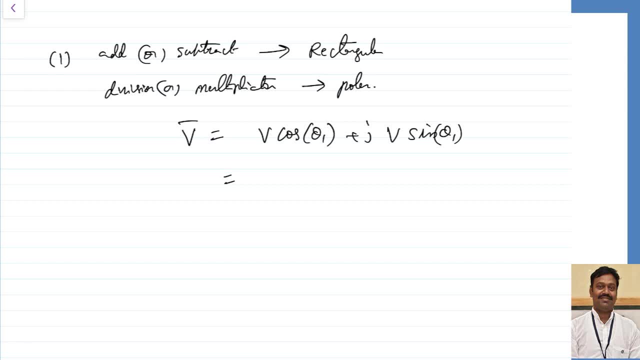 whereas in polar form. polar form will be represented by the magnitude with some angle: theta 1. so how can i calculate the angle theta 1? theta 1 is nothing but tan inverse of y component divided by x component. you have to remember this. so this way we have to do. so let us try to solve. 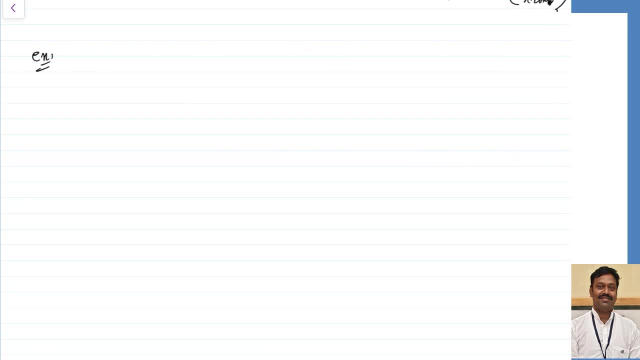 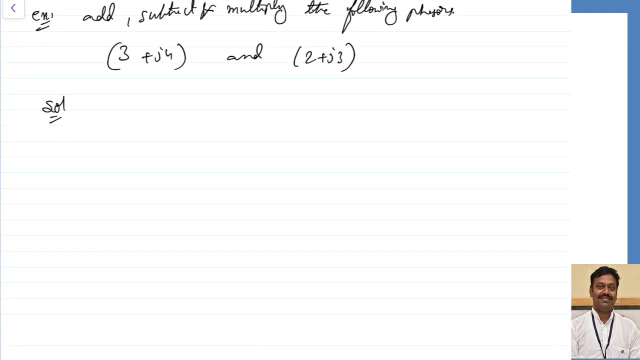 one or two numericals. so i am taking one more example: add, subtract and multiply the following phasors: so it is given there 3 plus j 4 and 2 plus j 3. so how to solve this? so this can be solved as i am just taking: a is equal. 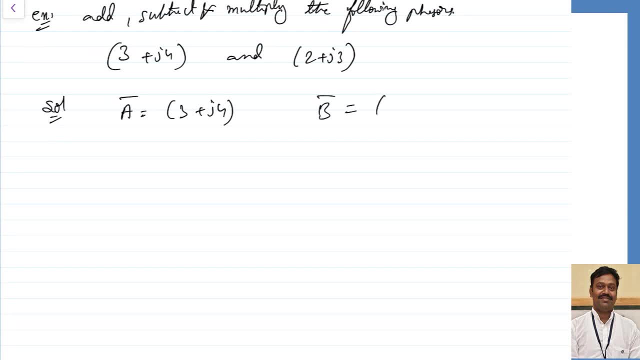 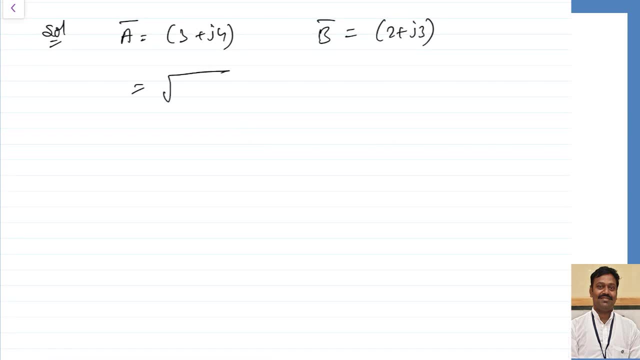 to 3 plus j 4 and i am taking b as 2 plus j 3. so when you are taking these two, so this i can convert to the polar form. so polar form will be equal to square root of 3 square plus 4 square. at an angle of tan inverse of y by x, y component is 4, x component. so this is: 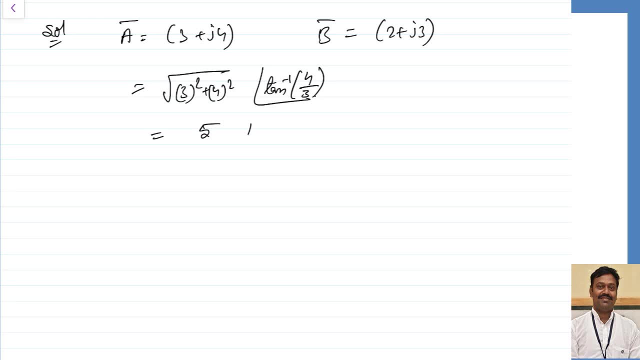 equal to 3 plus j 3. so if you calculate this you will get as 5 at an angle of 53.13 degrees. similarly, b i can calculate as square root of 2 square plus 3 square at an angle of tan inverse of y component by x component. so this will become 3.605 at an angle of 56.31. so 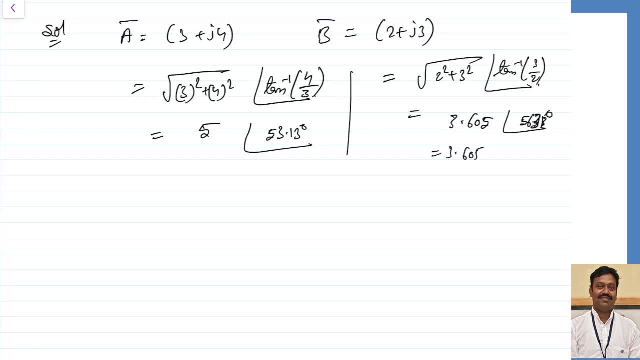 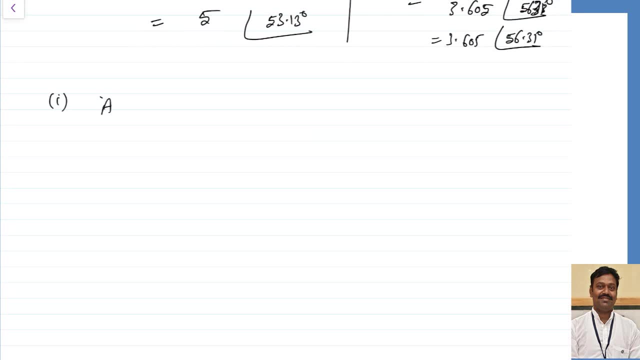 in this way you have to calculate. so i am just writing here: 3.605 at an angle of 56.31 degrees. so let us try to add. so i want to add the vector a plus vector b. i have told you that whenever addition is there, just doing the rectangular coordinate system, it is much. 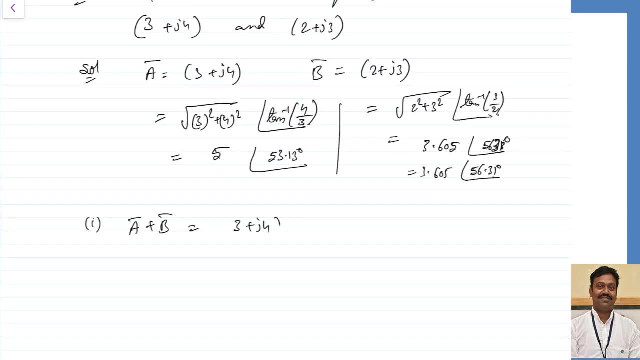 more easy, so in rectangular coordinate system. so i am just writing the values: plus 2 plus j, 3, so i have to just add the x component and the white component. so 3 plus 2 is 5, plus j of 4 plus 3 is 7.. 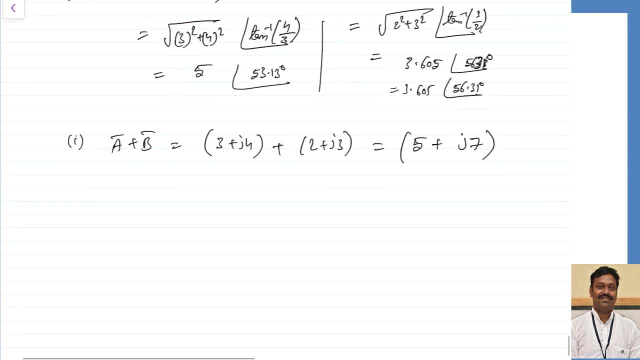 once i get this, i can convert to any other form easily. how to convert to other form in polar form will be equal to 5 square plus 7 square at an angle of tan inverse of 7 by 5. this way you can calculate. so if you calculate this, you will get this as 8.6 at an angle. 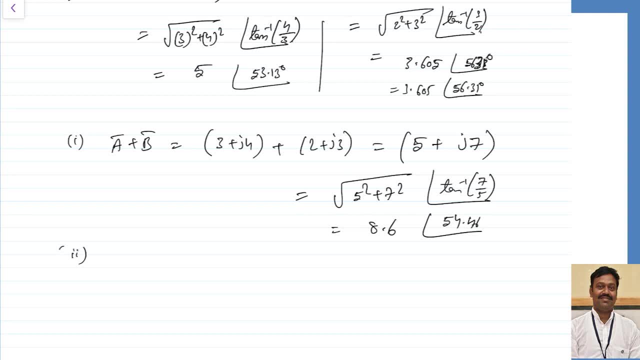 of 54.46. so similarly, if i want to calculate a minus b, a minus b is also easy: 3 plus j 4 minus 2 plus j 3. so 3 minus 2 becomes 1, and 4 minus j 3 becomes 1 and 4 minus j 3. 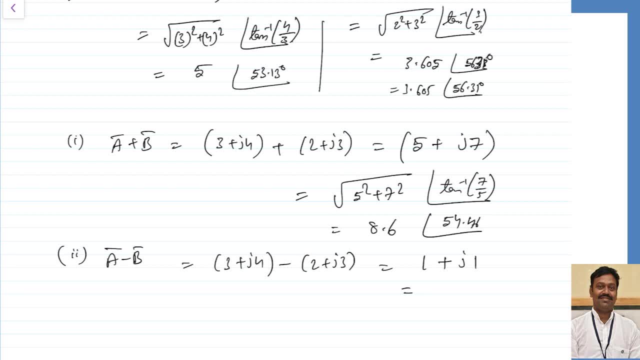 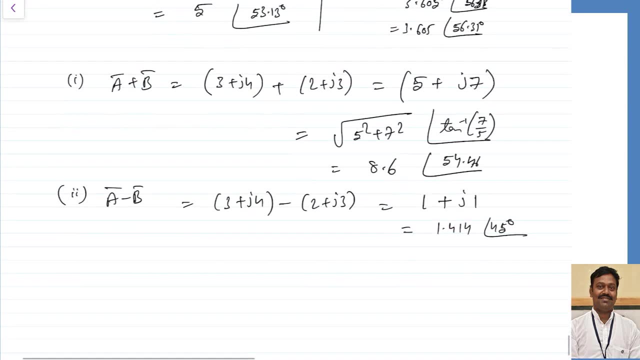 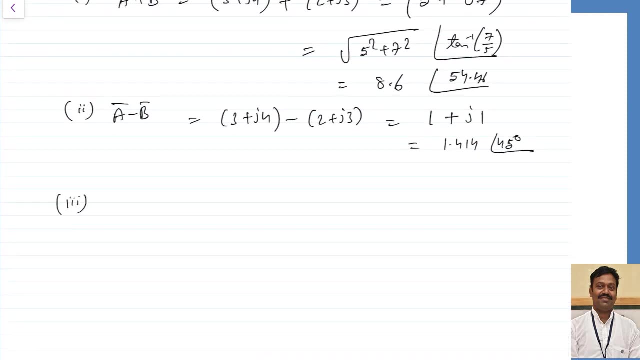 minus 3 becomes 1, 1 plus j, 1. so this i can convert to rectangular form 1.414 at an angle of 45 degrees. if you calculate this, a square plus b square and tan inverse of y component by x component. so now let us take, if i want to do the product of two, these two, so product. 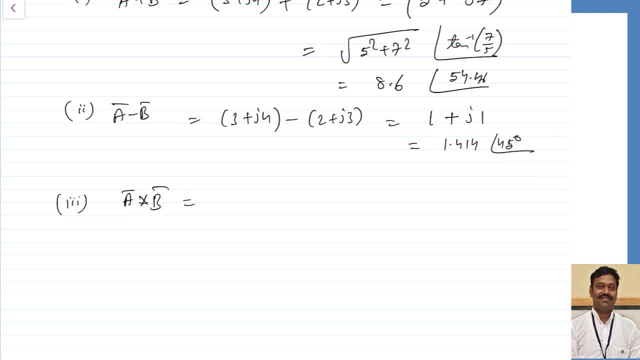 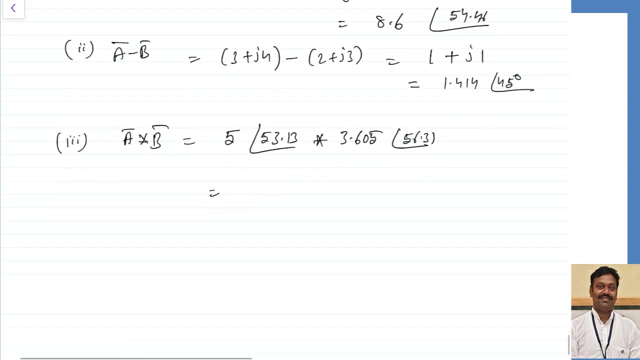 of these two. i told you, whenever you want to do the product, always go for polar coordinate system, because polar coordinate system is easy. so first one i can represent as 5 at an angle of 53.13.. just like that. next, multiply with 3.605 at an angle of 56.31. how to get this? you have to make the product. 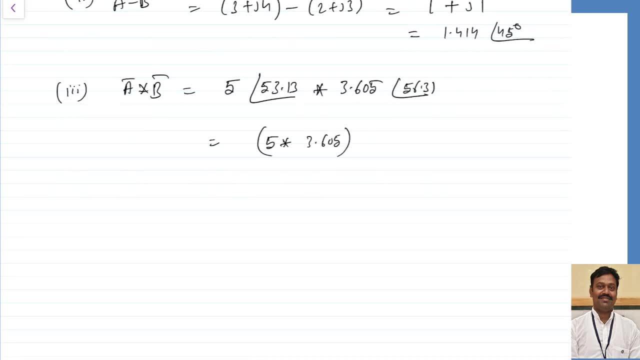 of the magnitudes and for angle should be added together, algebraically added together, so with their sign. so this way we have to add. fortunately here both are positive, so i am just directly adding: if one is negative, accordingly it will be subtracted, so this becomes 18.025 at an angle of 10.025. so this is the product of the magnitudes, and for angles should be added together, so this becomes 18.025 at an angle of 10.023.. So in this way we have to add. fortunately here both are positive, so i am just directly. 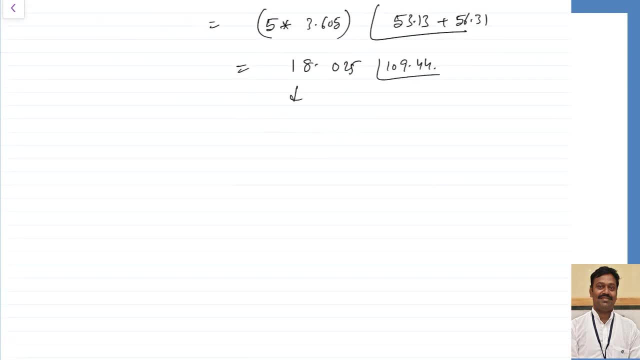 9.44.. Let us assume I want to convert this to rectangular form. How to convert this to rectangular form? So you have to multiply with cos 109 plus j times of the magnitude into sin of 109.44.. So if we calculate this, you will get it as 5.999 plus j, 16.997.. 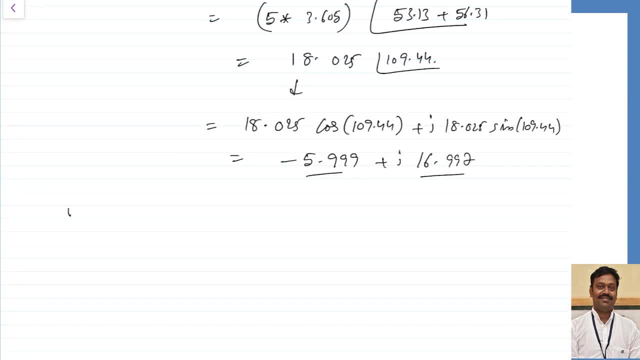 So this is what I got. Similar way, let us assume I want to divide the two phasors. If you want to divide the phasors also, it is very easy. in polar coordinate system, 3.605 at an angle of 56.31,. right What you have to do? you have to just divide the magnitudes. 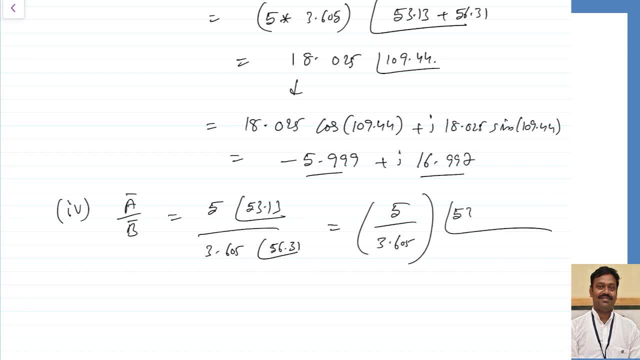 and angle should be subtracted from each other. So numerator minus whatever is there in the denominator, So you have to just subtract it. So if you subtract it you will get this value 5 by 3.605, 1.387 at an angle of minus 3.18 degrees. 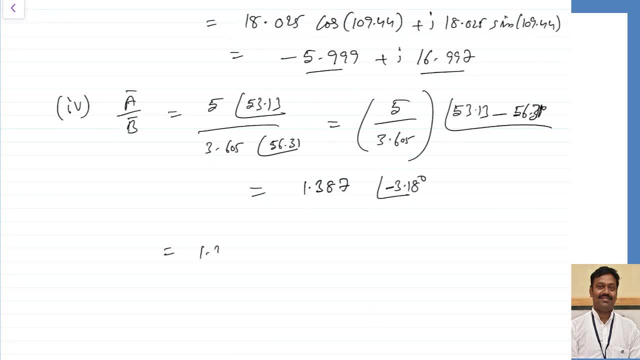 So how to convert this to rectangular form? So rectangular form will be 1.387 into cos of 3.18.. So here minus sign is there. So this will become minus j into 1.387, into sin of 3.18.. 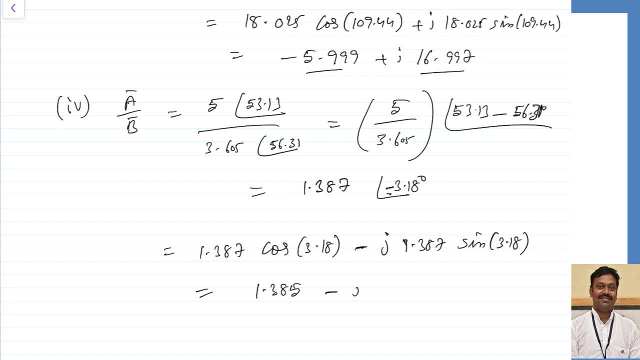 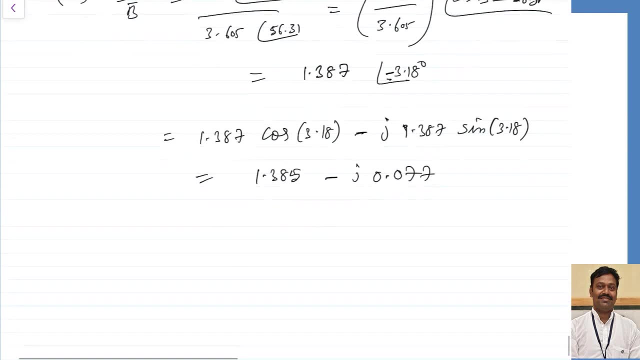 So if you substitute this 1.385, j 0.077.. Remember here this minus sign indicates that j will be minus, So remember that. I hope this is clear to you. So let us now proceed further, or if you are feeling confused: 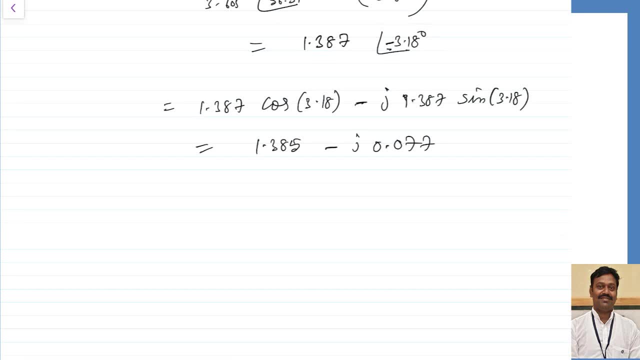 and just substitute the angle. only Just you can substitute the angle this: cos of minus 3.18, sin of minus 3.18. Just take plus j. That means you can take plus j and minus here. In that case also you will get it same. if you are having the confusion Getting it, Let us take one more small. 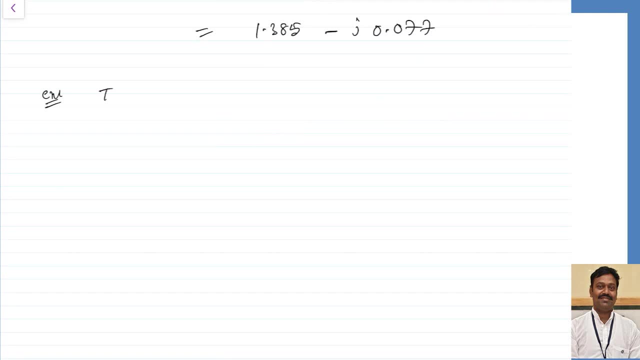 numerical so that this concept will be completely clear. So let us take one more small numerical so that this concept will be completely clear. So let us take one more small numerical so that this concept will be completely clear to you. So it is given. 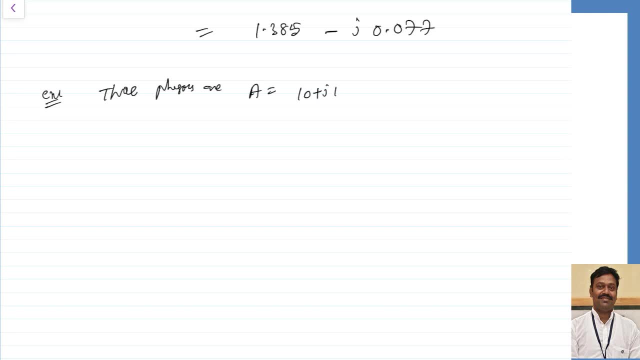 Three phasors are: a is equal to 10 plus j 10,, b is equal to 50 at an angle of 120 degrees and c is equal to 8 minus j 6. It is given like this and it is asked: evaluate a, b by c and express in: 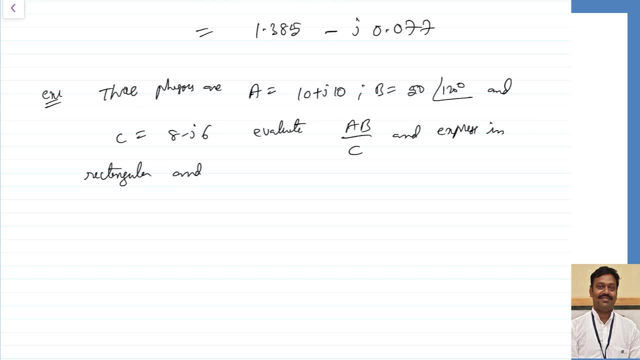 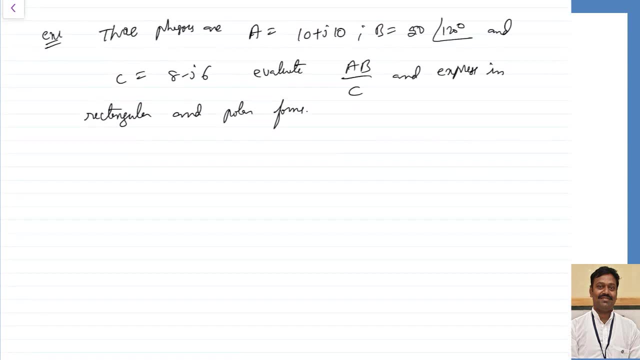 So it is given like this and it is asked: evaluate a, b by c and express in rectangular and polar forms. This is what is asked. So three are given there. So, first thing, what I have to do, just try and write them and convert to the second form so that the calculation will be. 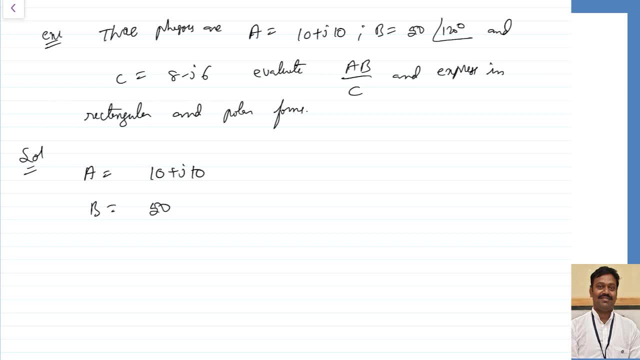